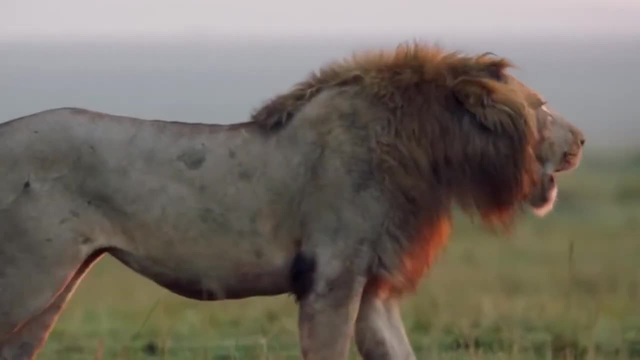 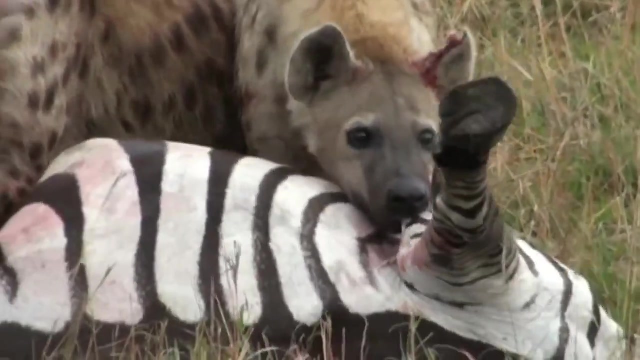 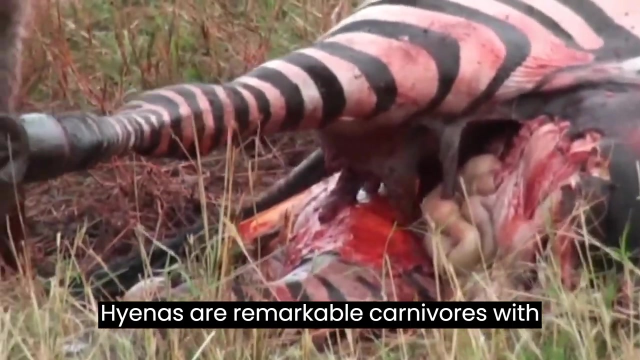 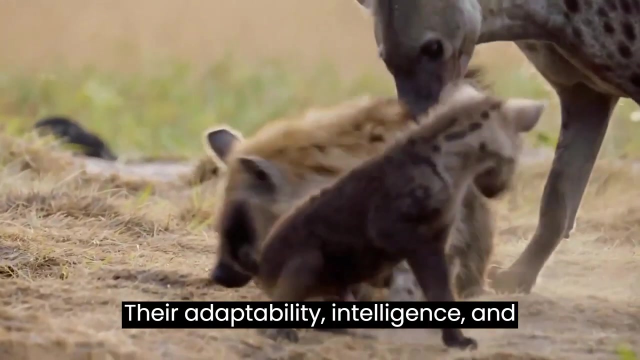 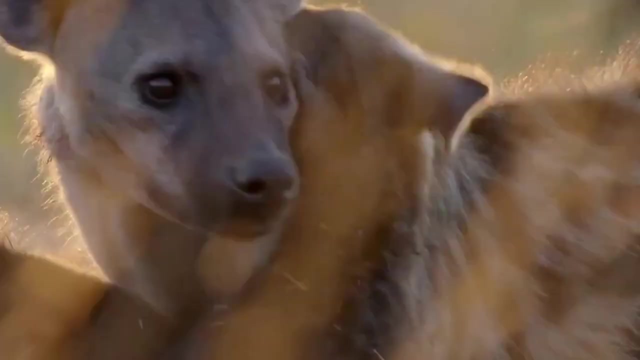 Hyenas are remarkable carnivores with unique social structures, communication methods and hunting strategies. Their adaptability, intelligence and cooperative behavior contribute to their success in a variety of environments. Whether hunting in coordinated groups or scavenging for carrion, hyenas play a crucial 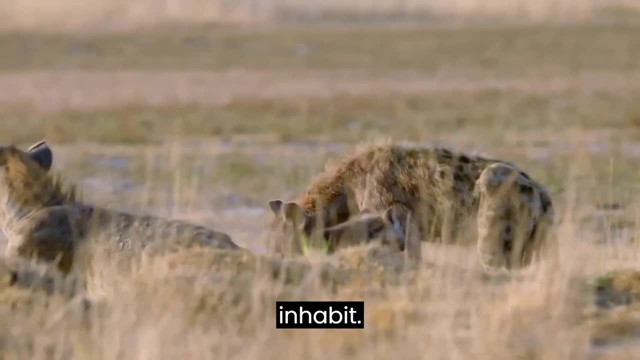 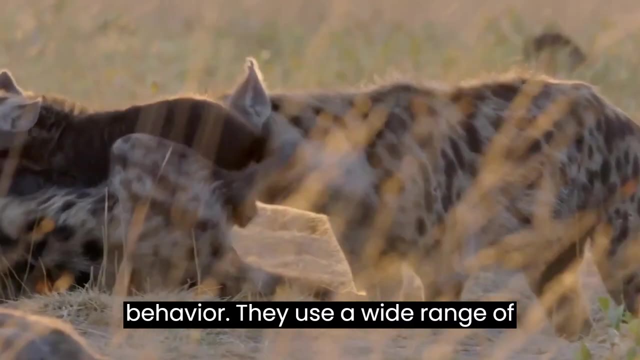 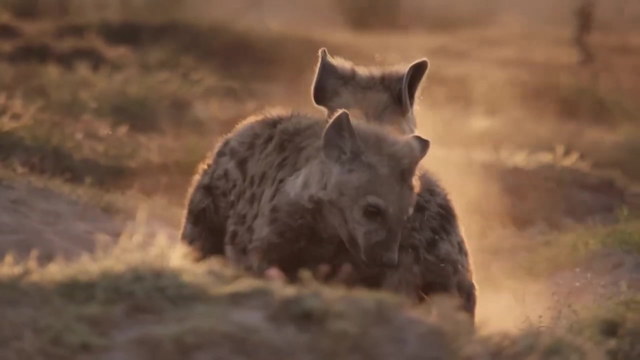 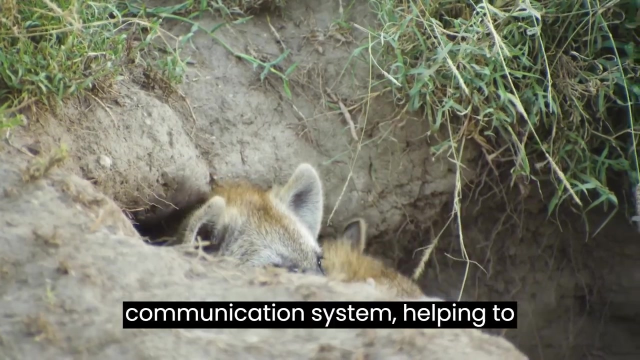 role in maintaining the ecological balance of the ecosystems they inhabit. Communication is a key aspect of hyena behavior. They use a wide range of vocalizations, including whoops, growls and distinctive laughter-like calls, to communicate with clan members. Marking visual signals and body language also contribute to their complex communication. 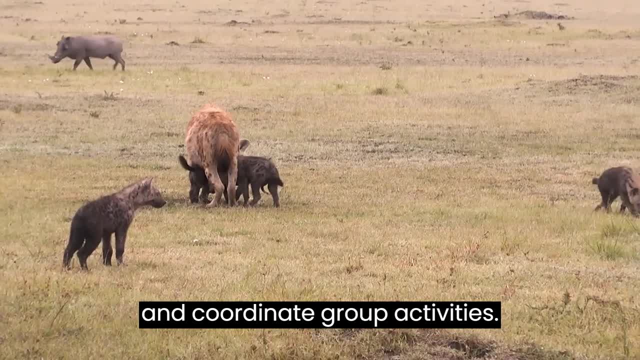 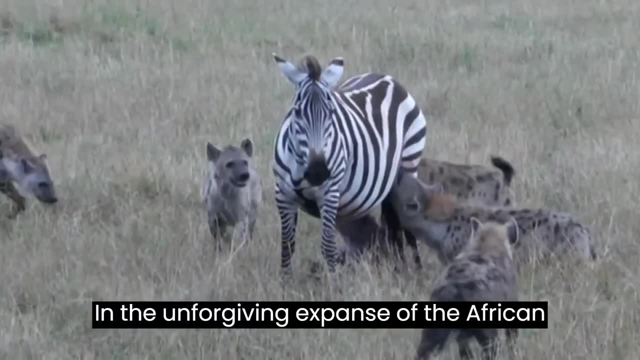 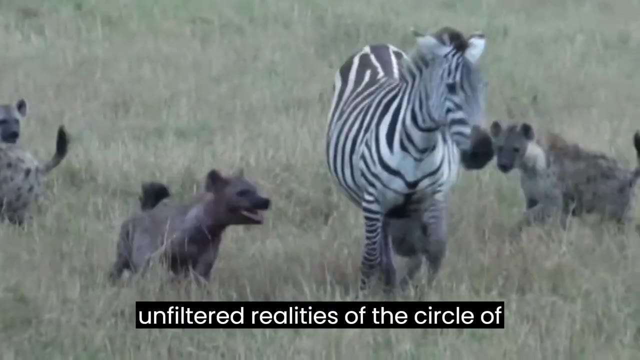 system, helping to establish territory, convey dominance and coordinate group activities. In the unforgiving expanse of the African savannah, a stark and brutal tableau unfolds, showcasing the raw and unfiltered realities of the circle of life: A group of hyenas. 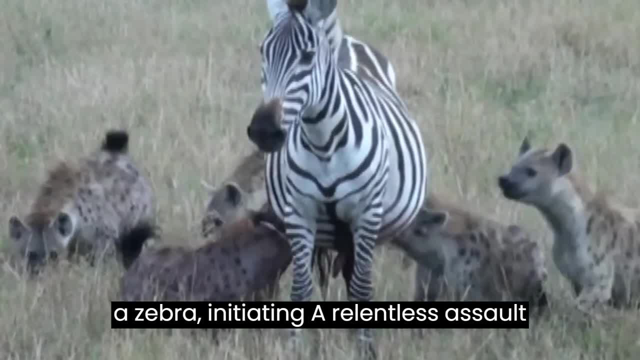 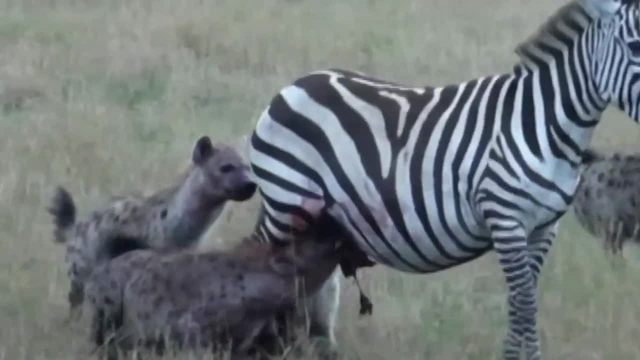 renowned for their relentless hunting prowess, descends upon a zebra, initiating a relentless assault that echoes the primal instincts of survival inherent in the natural world. The zebra's attempts are futile and its once-powerful legs betray it under the overwhelming force. 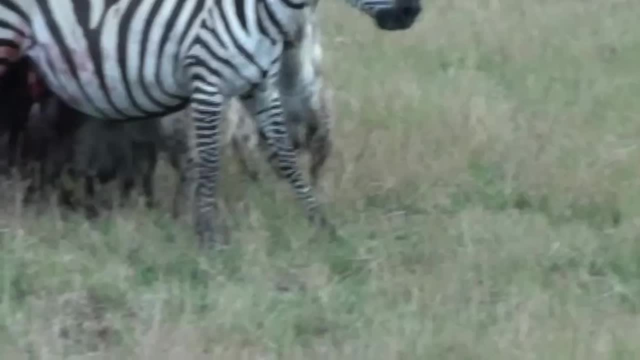 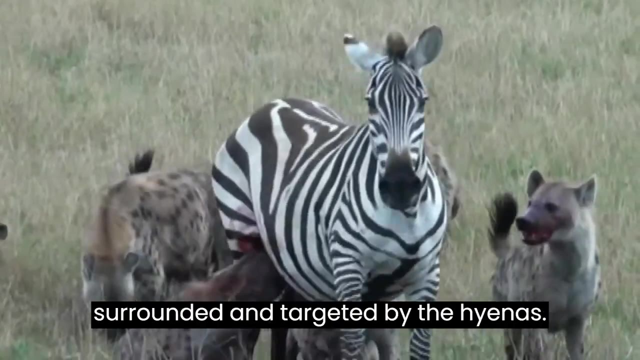 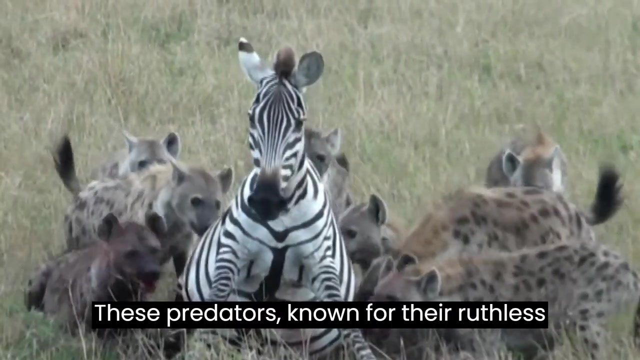 of the hyena's bites, Once a symbol of grace and vitality. against the sprawling backdrop of the savannah, the striped equine finds itself surrounded and targeted by the hyenas. These predators, known for their ruthless efficiency, converge on the zebra from all 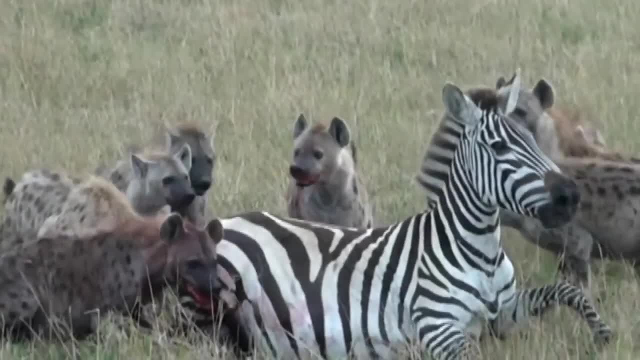 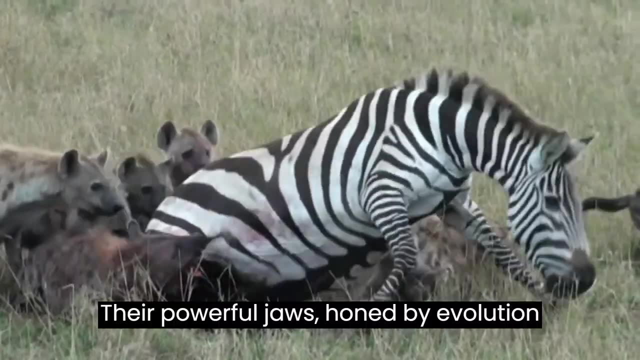 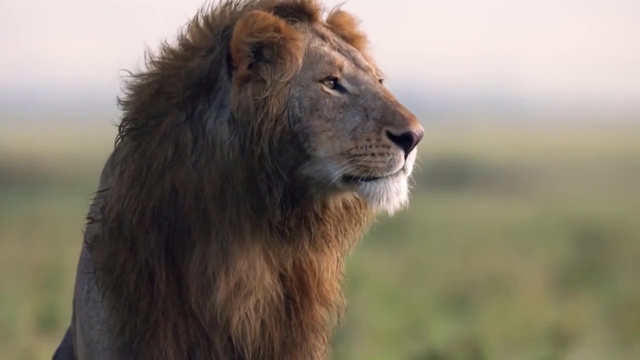 sides, orchestrating a coordinated attack. Their powerful jaws, honed by evolution for tearing through flesh and bone, become instruments of predation in a calculated effort to subdue their prey. On the other hand, a captivating scene unfolds as a group of hyenas converges around a solitary 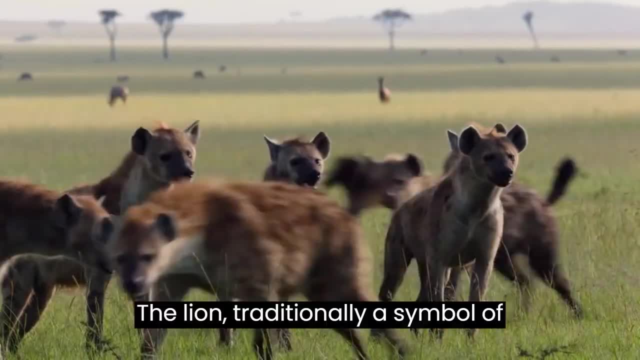 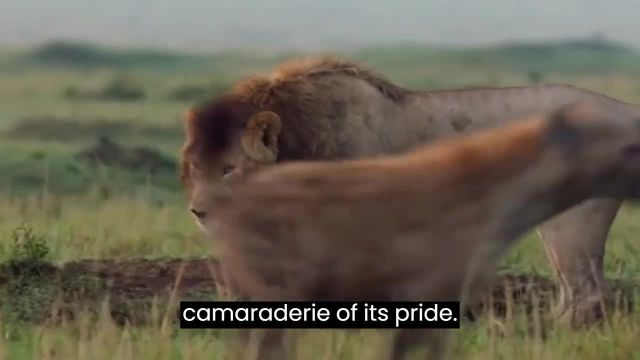 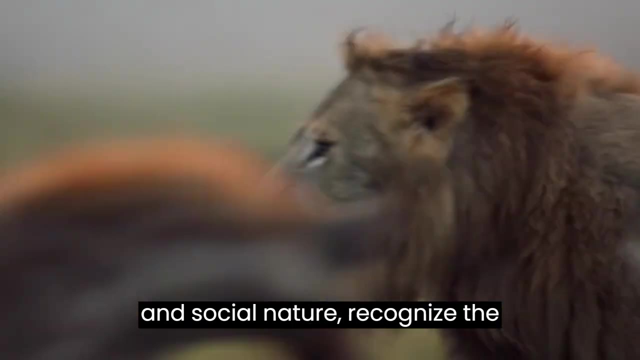 lion that finds itself separated from its pride. The lion, traditionally a symbol of regality and power in the animal kingdom, stands alone, away from the safety and camaraderie of its pride. The hyenas, known for their opportunistic and social nature, recognize the vulnerability. 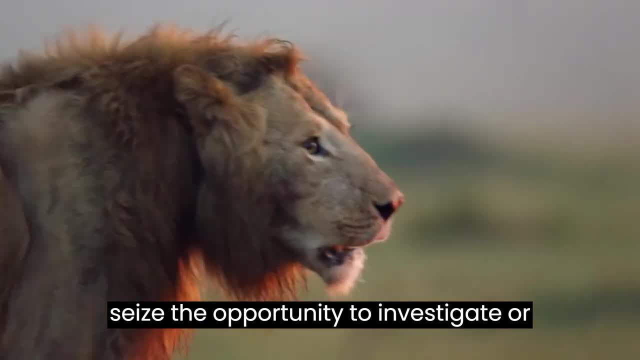 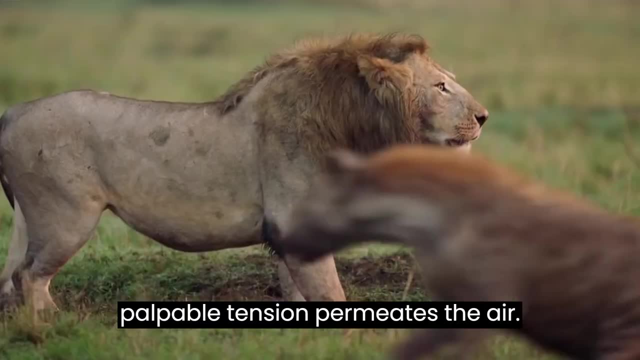 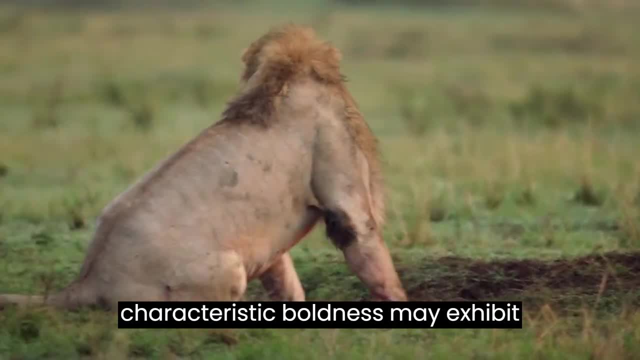 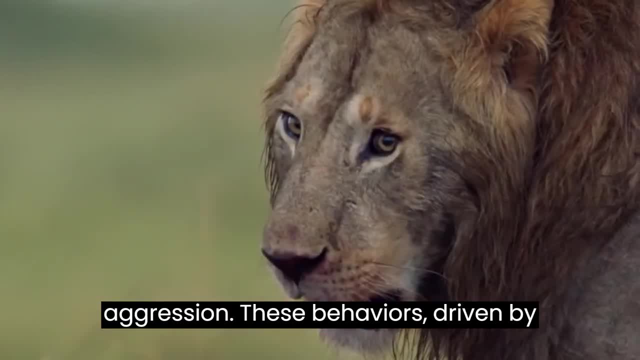 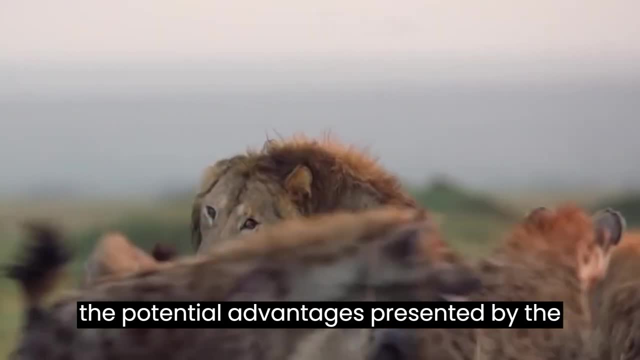 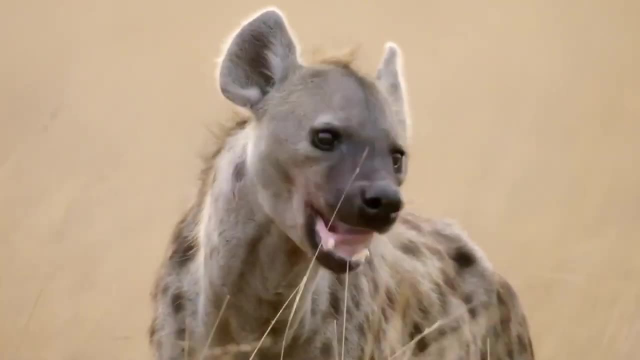 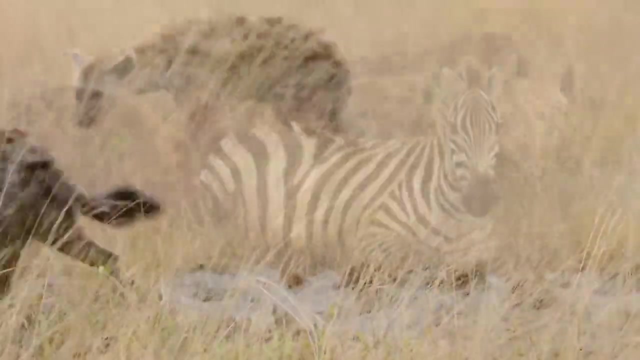 curiosity to aggression. These behaviors, driven by a mix of curiosity and opportunism, illustrate the hyena's keen awareness of the potential advantages presented by the lone lion. As the assault intensifies, the zebra attempts to flee in a desperate bid to escape the relentless 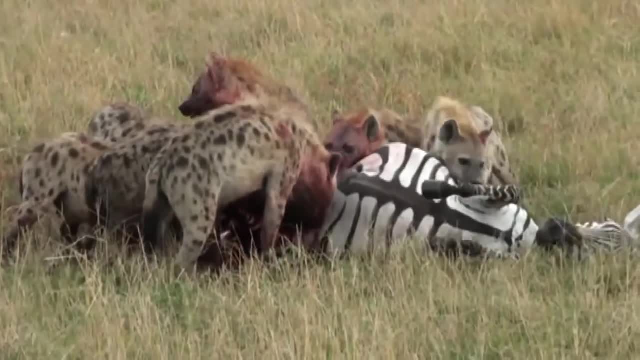 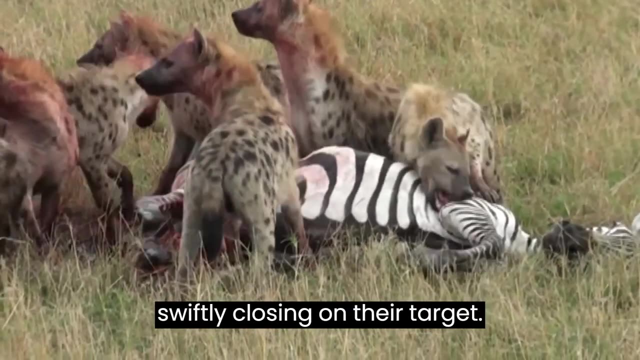 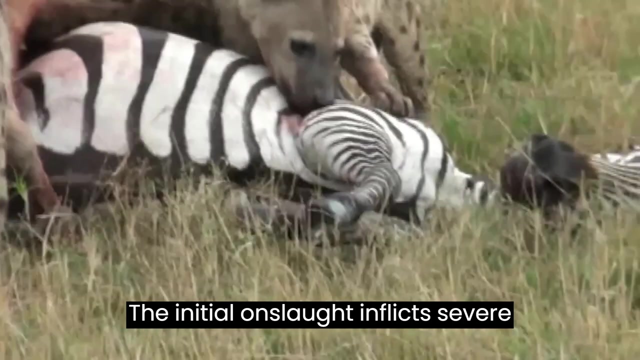 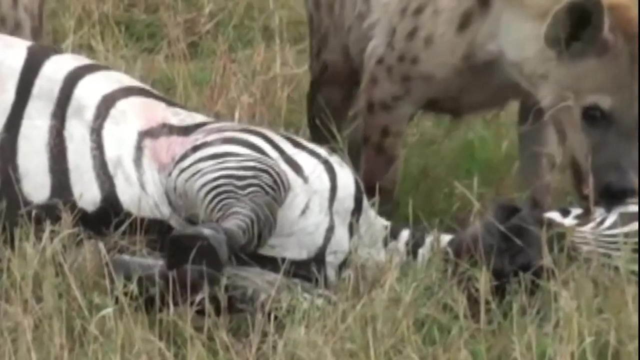 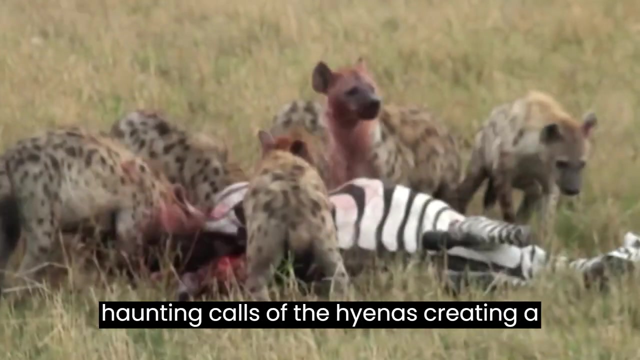 onslaught. However, the hyenas, displaying their cunning tactics and numerical advantage, swiftly close in on their target. The initial onslaught inflicts severe injuries upon the zebra, rendering it helpless and incapacitated. The air resonates with the distressing sounds of the struggle, punctuated by the haunting. 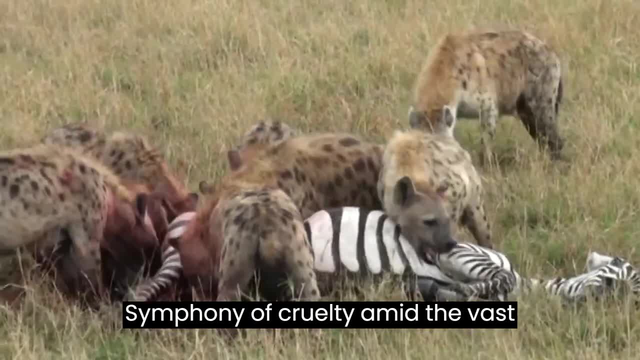 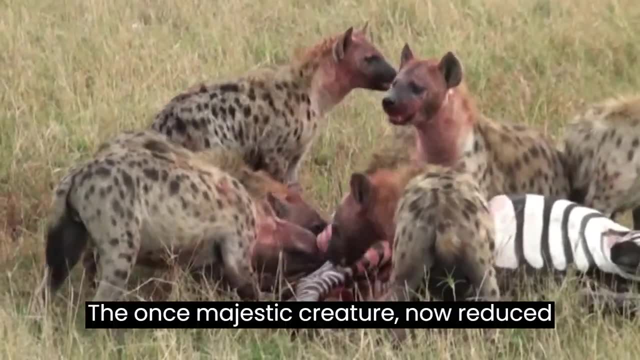 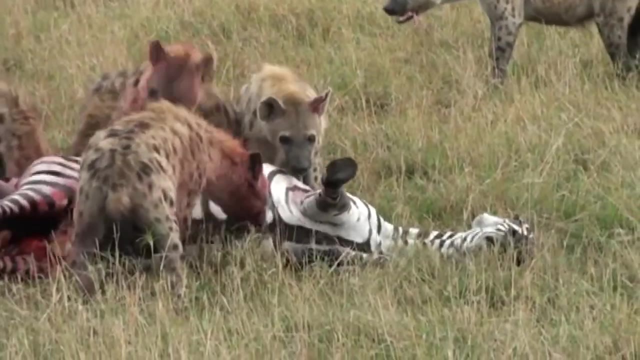 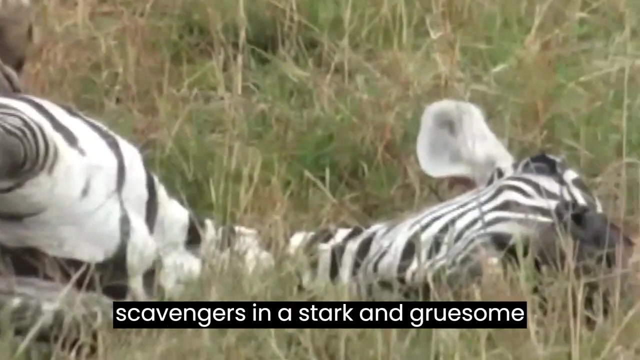 calls of the hyenas, creating a symphony of cruelty. amid the vast savannah, The once majestic creature, now reduced to a weakened and vulnerable state, struggles in vain to free itself from the unyielding grip of the hyenas. The hyenas transition from hunters to scavengers in a stark and gruesome display of nature's. 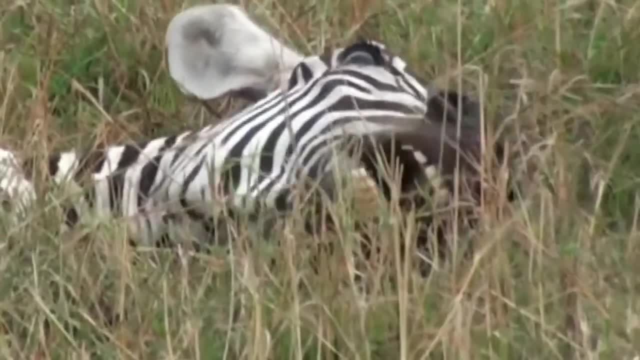 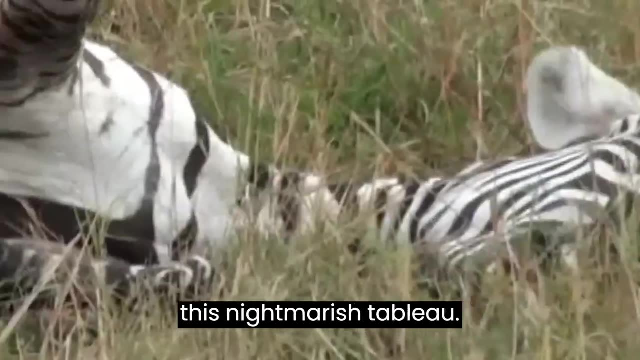 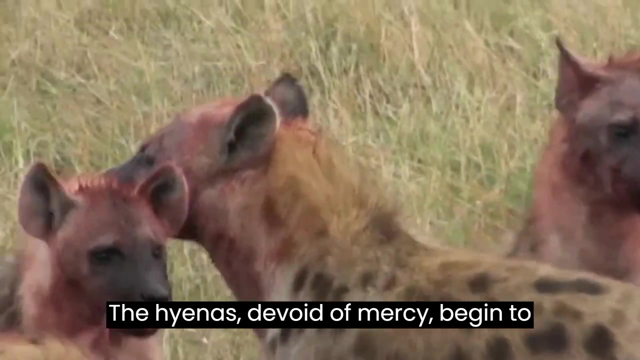 brutality. The zebra, still alive and conscious, becomes the unfortunate centerpiece of this nightmarish tableau. The hyenas, devoid of mercy, begin to feed on the still-living creature, tearing into its flesh with a disturbing lack of control. 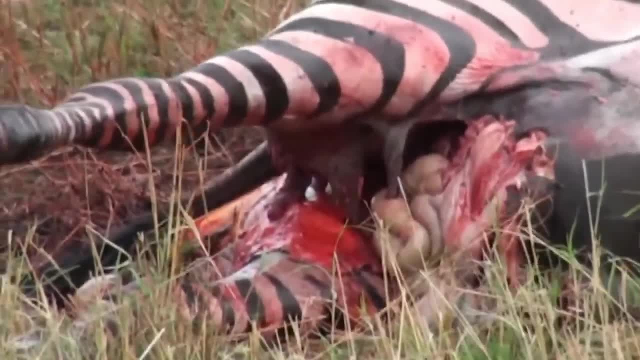 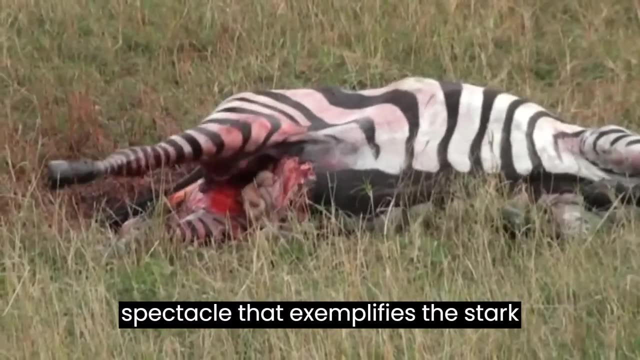 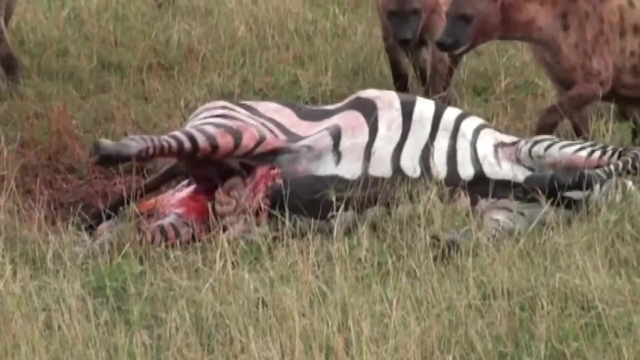 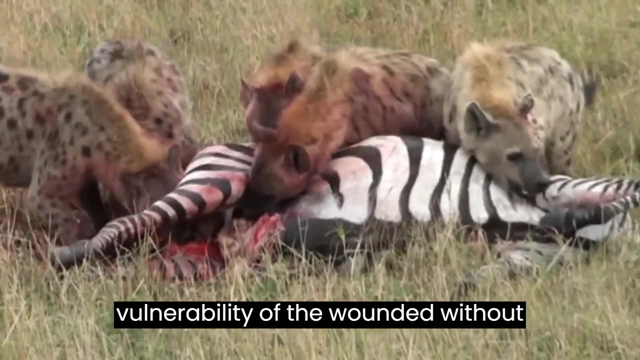 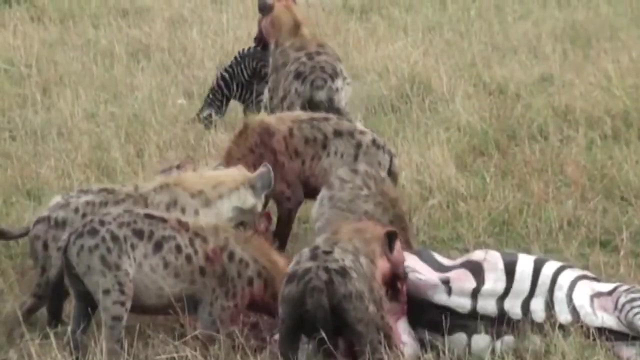 remorse. The scene unfolds as an agonizing spectacle that exemplifies the stark reality of the circle of life in the wild, Predators, driven by the relentless pursuit of prey for survival, exploit the vulnerability of the wounded without sentiment. The savannah, although breathtakingly beautiful, reveals its unforgiving nature where life 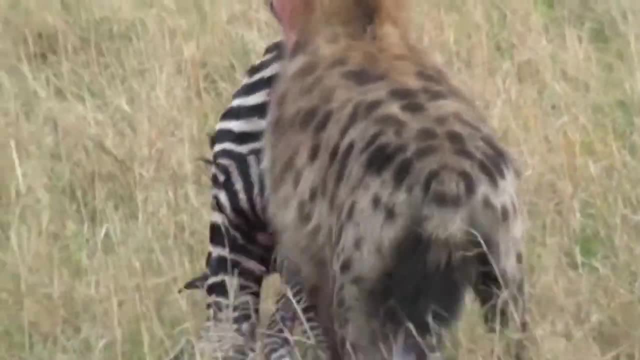 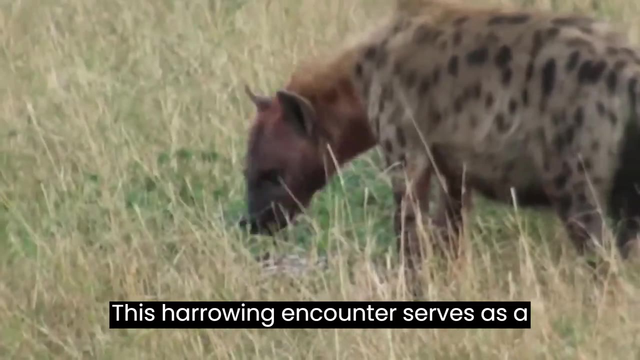 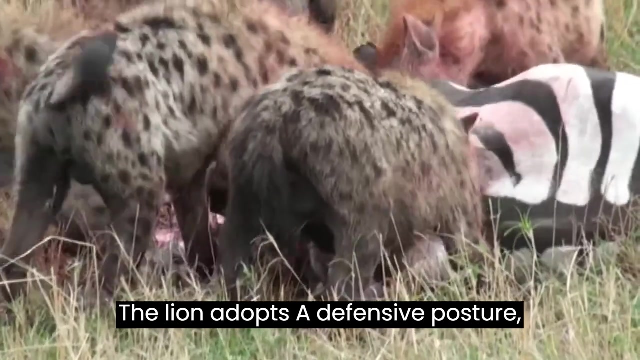 and death coexist in a relentless dance of primal instincts. This harrowing encounter serves as a poignant reminder of life's intricate dynamics and inherent harshness. in the wild, The lion adopts a defensive posture. The lion adopts a defensive posture watching the encircling hyenas, while occasionally emitting. 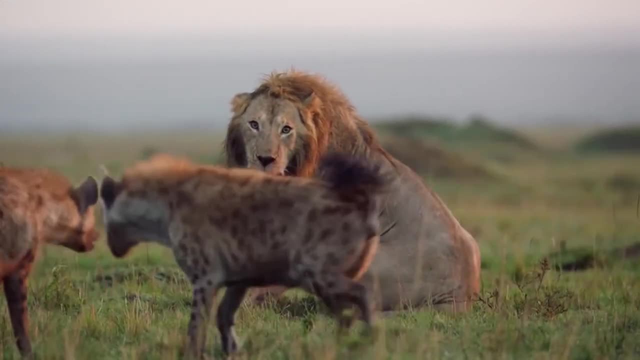 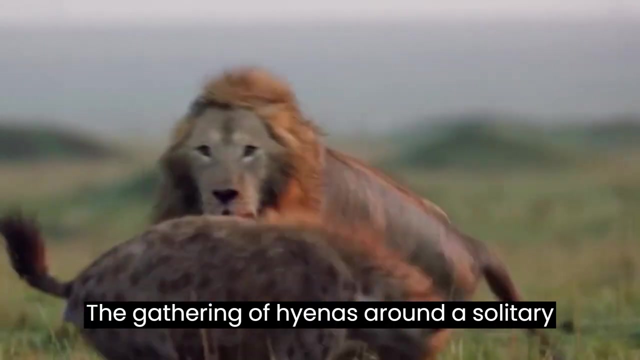 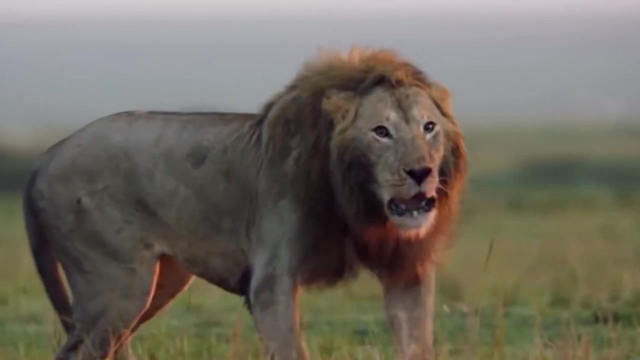 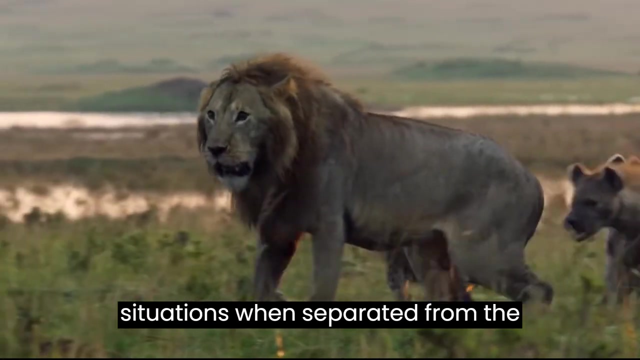 warning growls or threatening gestures. The gathering of hyenas around a solitary lion reflects the perpetual dance of power hierarchy and survival. in the savannah ecosystem. Lions are apex predators, but even they can find themselves in precarious situations when separated from the protective umbrella of their prey. 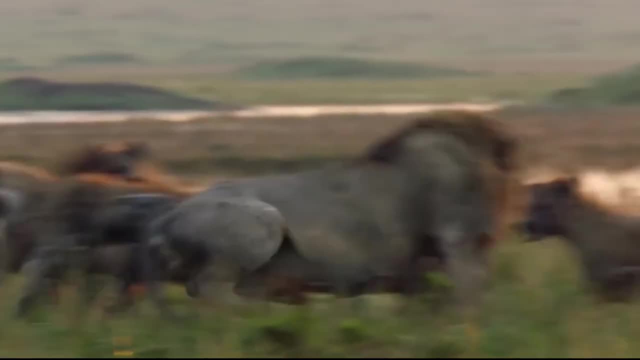 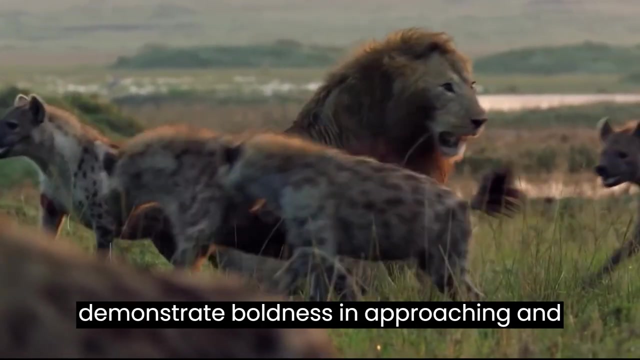 Lions are apex predators, but even they can find themselves in precarious situations when separated from the protective umbrella of their prey. lord 숙, sergeant sergeant With her numbers and cooperative hunting strategies, hyenas often demonstrate boldness in approaching and testing larger predators, especially when the odds are in their favor. 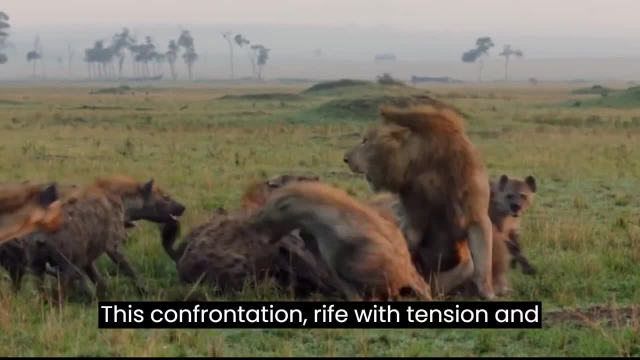 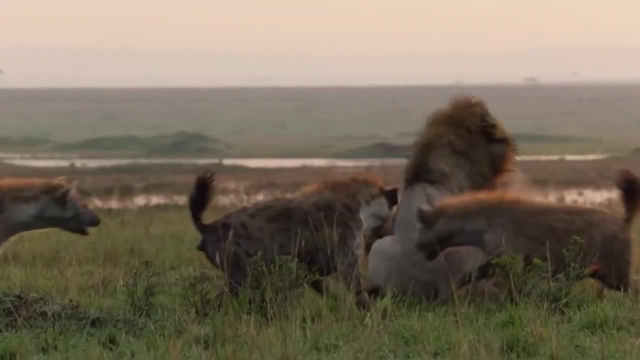 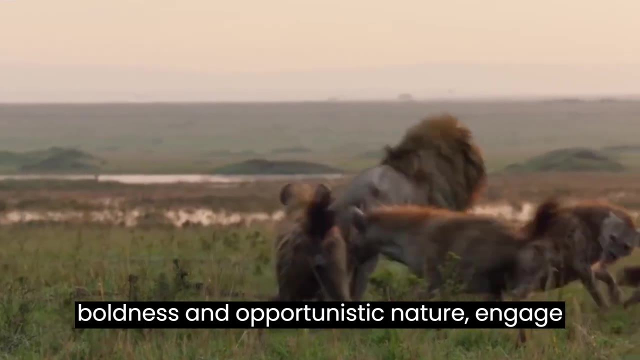 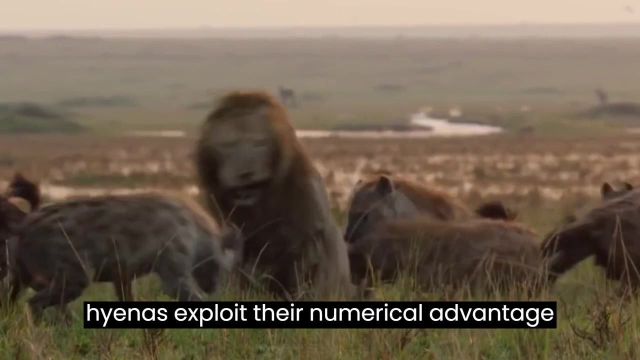 serian ball Two-headed hunter, piel 住 wild sea lion- lion. boldness and opportunistic nature engage in a relentless assault on the lion, Nipping at its flanks and testing the boundaries of the big cat's endurance, the hyenas exploit their numerical 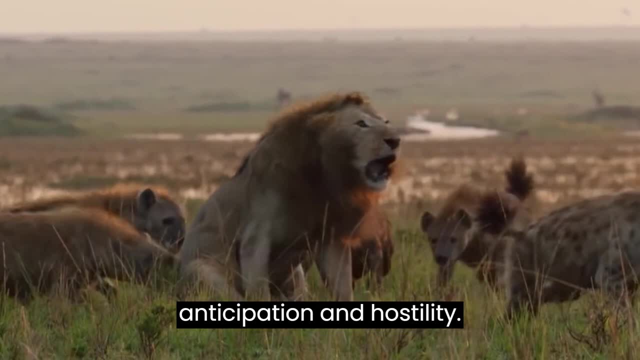 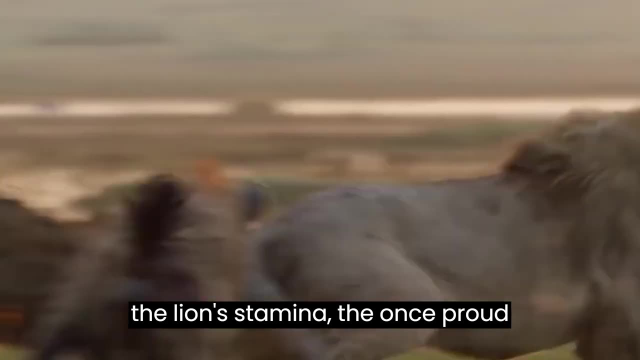 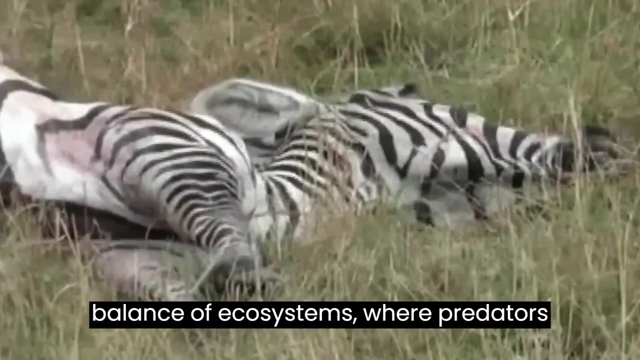 advantage to create a charged atmosphere thick with anticipation and hostility. As the relentless harassment wears down the lion's stamina, the once-proud creature valiantly attempts to fend off the persistent attackers. It prompts contemplation on the delicate balance of ecosystems where predators and prey engage in a perpetual struggle for survival.